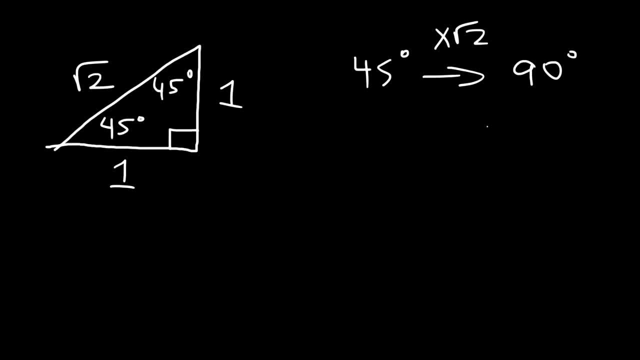 If you have the side that's across the 90-degree angle and you want to calculate the length of the side across the 45-degree angle, you need to divide by the square root of 2.. So I'm going to put this into practice and show you how to apply this information. 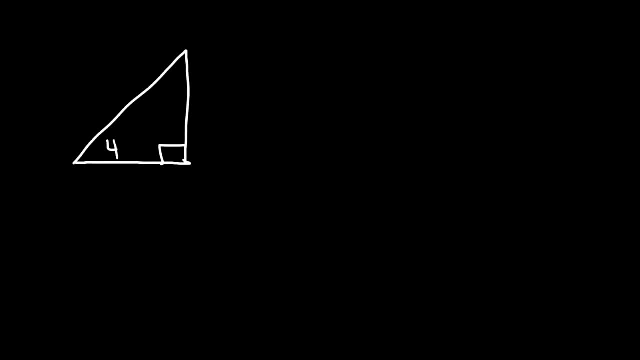 So consider this right triangle and you're given the length of one of the legs of the right triangle, 5'2". Find the missing two sides. Well, we know this is a 45-45-90-degree triangle, so these two sides have to be the same. 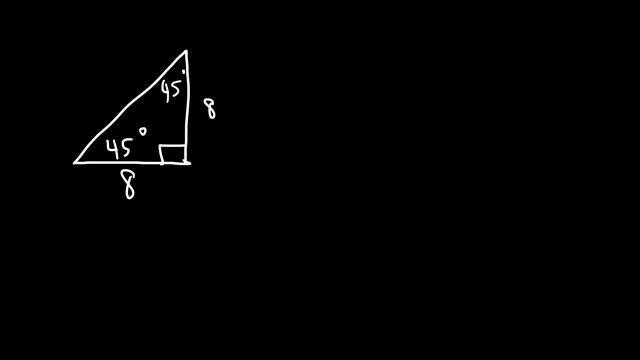 So if the bottom leg is 8, the other one is 8.. Now to find the hypotenuse, which is always the longer side, we have to multiply this side by the square root of 2.. So this is going to be 8, square root 2.. 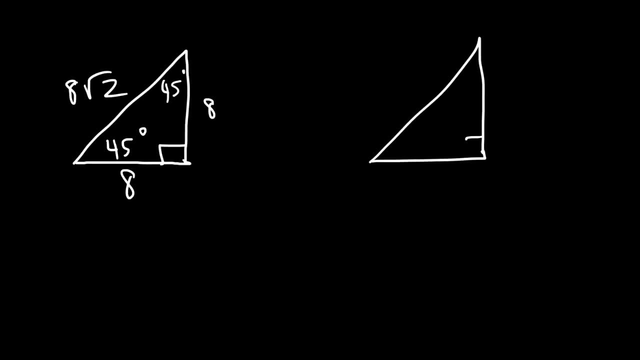 So, based on that example, feel free to pause the video and try this example. Go ahead and find the missing sides. So the other side is 12 units long and the hypotenuse is going to be: this number times the square root of 2.. 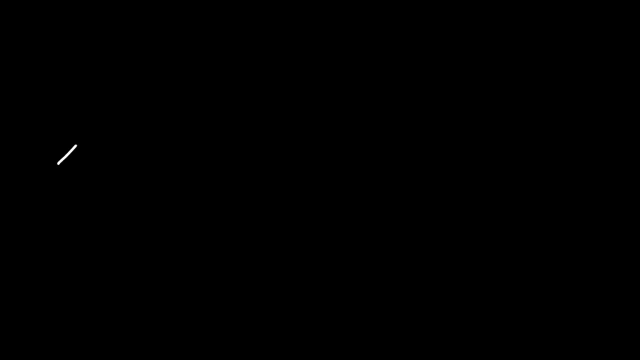 So it's 12 roots of 2.. Now go ahead and try these two examples. So let's say that this side is 5, square root 2, and here's another one, And let's say this side is 7, square root 2.. 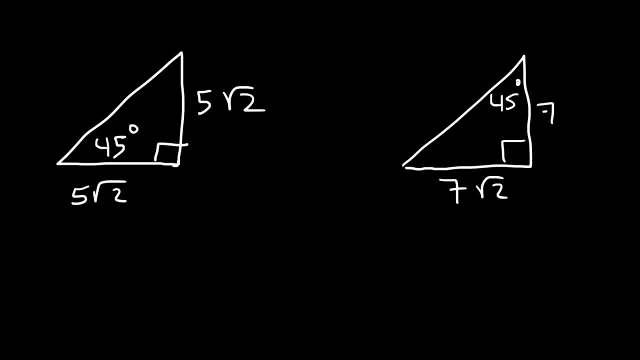 So we know the other missing side has to be the same. That's not going to change. Now let's find the hypotenuse of the first triangle. So we've got to multiply it by square root 2 if we want to find the length of the hypotenuse. 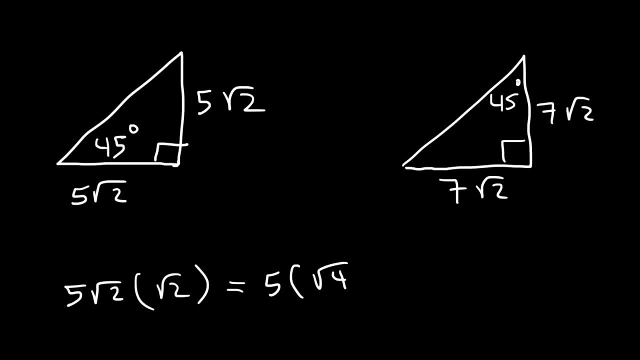 So the square root of 2 times the square root of 2 is the square root of 4.. And the square root of 4 is 2.. And 5 times 2 is 3.. And 5 times 2 is 10.. 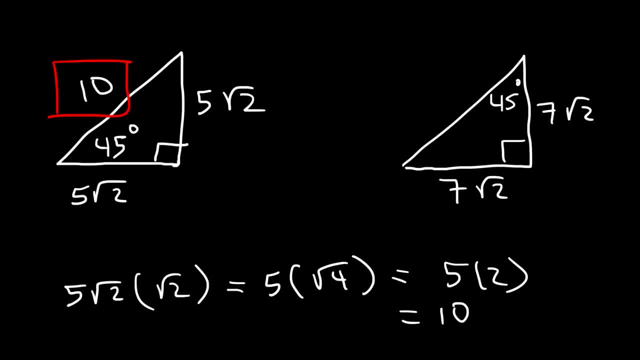 So the hypotenuse is 10 units long And it's very easy to find the missing side if you understand this particular special reference triangle, So let's do the same thing for this one. So if we multiply 7 square root 2 by the square root 2, this is going to be 7 times 2, which ends up being 14.. 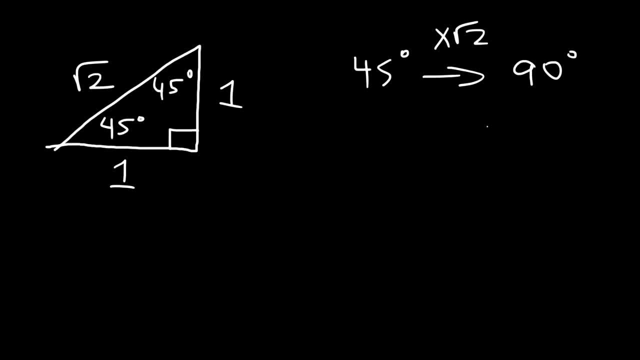 If you have the side that's across the 90-degree angle and you want to calculate the length of the side across the 45-degree angle, you need to divide by the square root of 2.. So I'm going to put this into practice and show you how to apply this information. 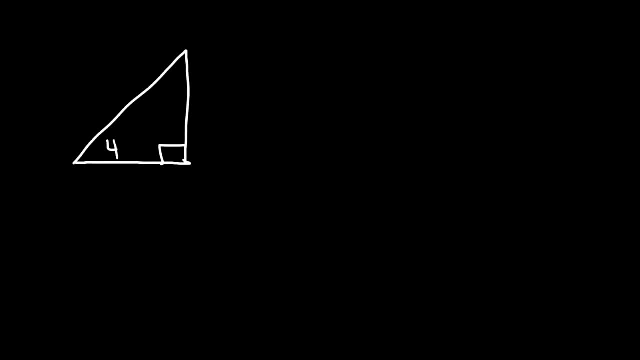 So consider this right triangle and you're given the length of one of the legs of the right triangle, 5'2". Find the missing two sides. Well, we know this is a 45-45-90-degree triangle, so these two sides have to be the same. 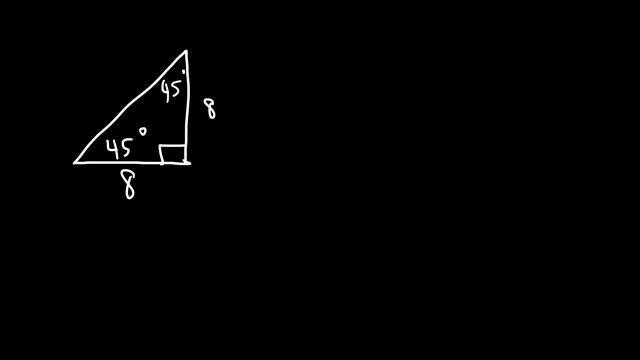 So if the bottom leg is 8, the other one is 8.. Now to find the hypotenuse, which is always the longer side, we have to multiply this side by the square root of 2.. So this is going to be 8, square root 2.. 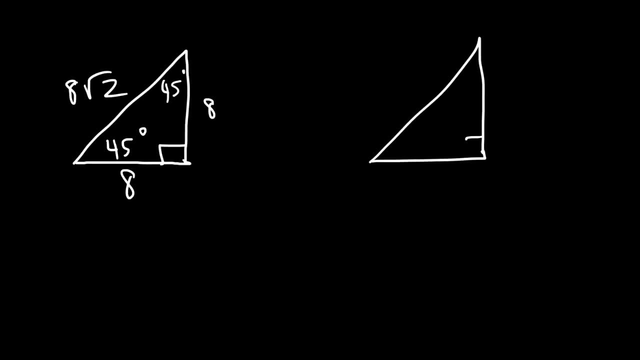 So, based on that example, feel free to pause the video and try this example. Go ahead and find the missing sides. So the other side is 12 units long and the hypotenuse is going to be: this number times the square root of 2.. 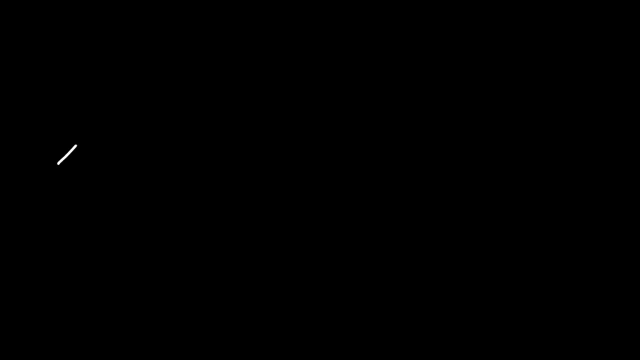 So it's 12 root 2.. Now go ahead and try these two examples. So let's say that this side is 5 square root 2, and here's another one. And let's say this side is 7 square root 2.. 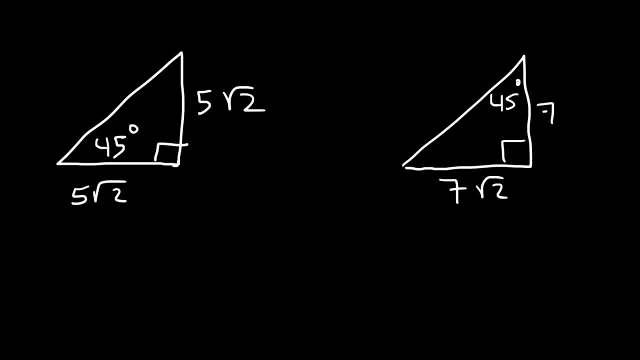 So we know the other missing side has to be the same. That's not going to change. Now let's find the hypotenuse of the first triangle. So we've got to multiply it by square root 2 if we want to find the length of the hypotenuse. 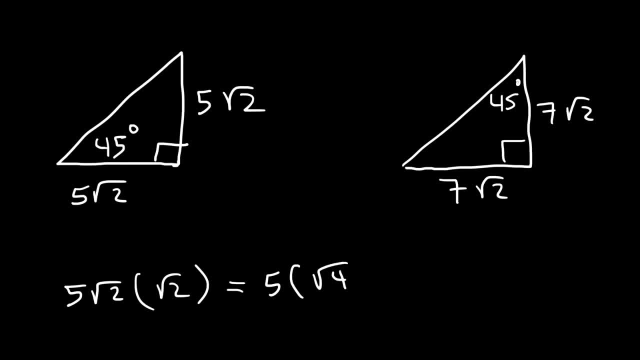 So the square root of 2 times the square root of 2 is the square root of 4.. And the square root of 4 is 2.. And 5 times 2 is 3.. So the hypotenuse is 10 units long. 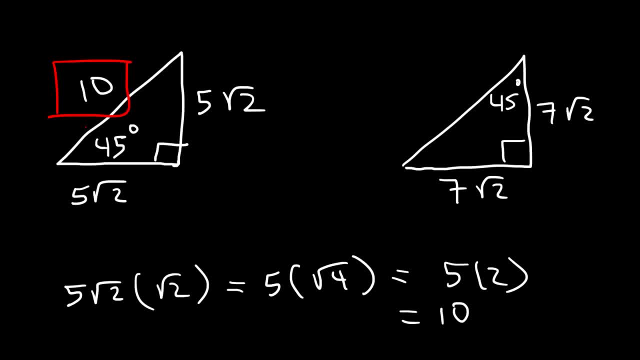 And it's very easy to find the missing side if you understand this particular special reference triangle. So let's do the same thing for this one. So if we multiply 7 square root 2 by the square root 2, this is going to be 7 times 2, which ends up being 14.. 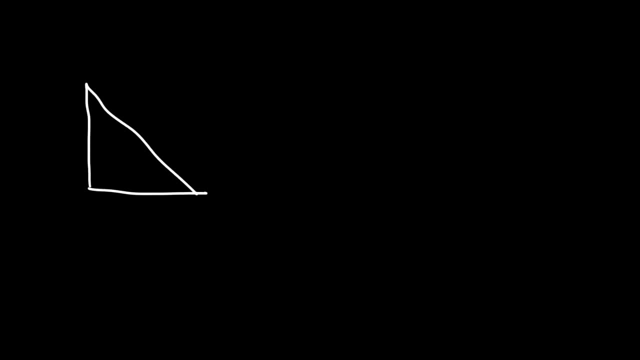 So let me give you some other examples. Let's change it up a little. So this time you're given the hypotenuse. Go ahead and find the value of the missing sides of these two triangles. Now, this time we have the side across the 90 degree angle, which is basically the hypotenuse. 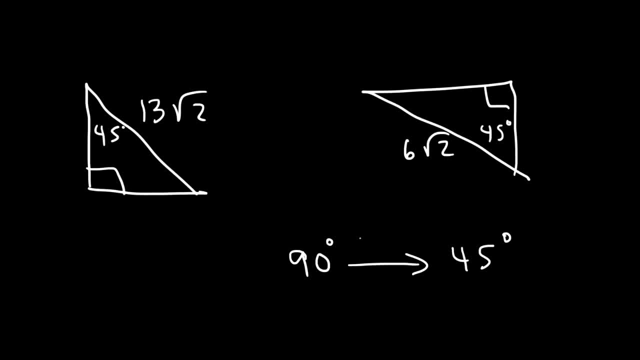 And we want to find the side across the 45. So we're looking for the value of the shortest side. So we need to divide by the square root of 2.. So if we take the hypotenuse 13 square root 2, and divide it by the square root 2,, 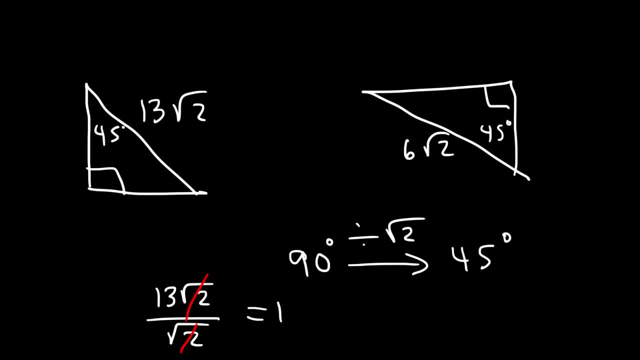 these two will cancel and we're just going to get 13.. So the length of these two sides is 13.. Now if we do the same thing for the example on the right, if we take 6 square root 2, divide it by that, well that's going to give us 6.. 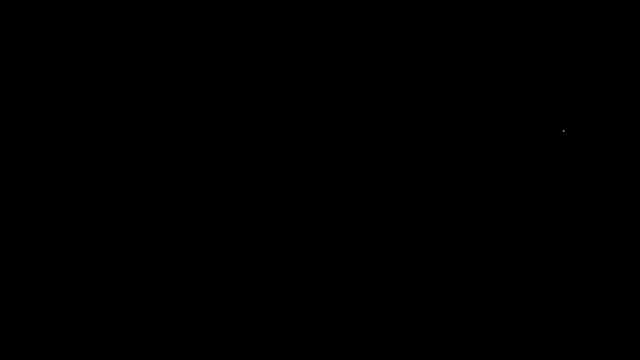 And so that's how we can easily find the value of the missing side. So consider these two examples. So let's say, this time the hypotenuse is 10, and for this one it's, let's say, 15.. Go ahead and calculate the value of the missing sides. 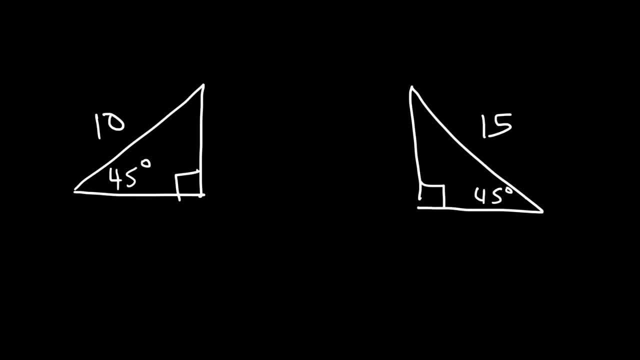 So we know, if we're given the hypotenuse to find the legs of the triangle, we've got to divide by the square root of 2.. So 10 divided by the square root of 2, is something that we need to rationalize. 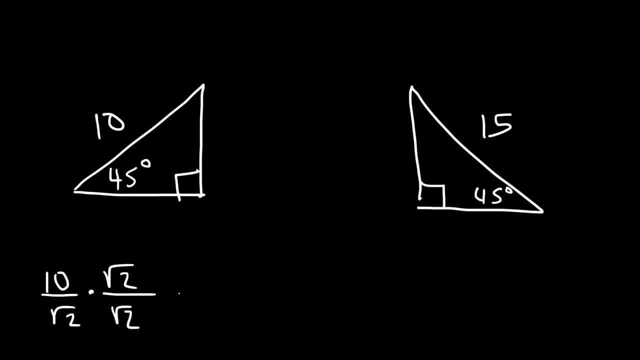 So let's multiply the top and the bottom by the square root of 2.. So on top we're going to have 10 square root 2, and on the bottom, the square root of 2 times the square root of 2 is 2.. 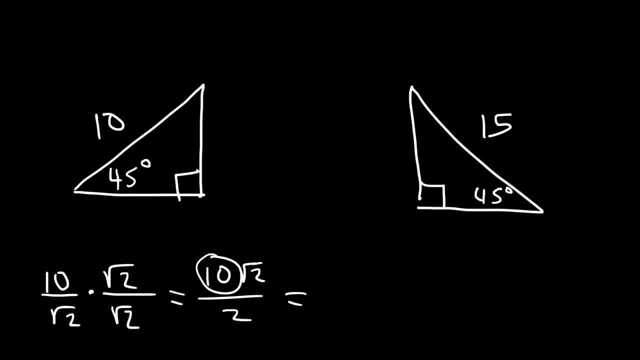 And so we could divide 10 by 2, which will give us 5.. So this is going to be 5 square root 2, and 5 square root 2.. Now let's do the same thing for the other triangle. 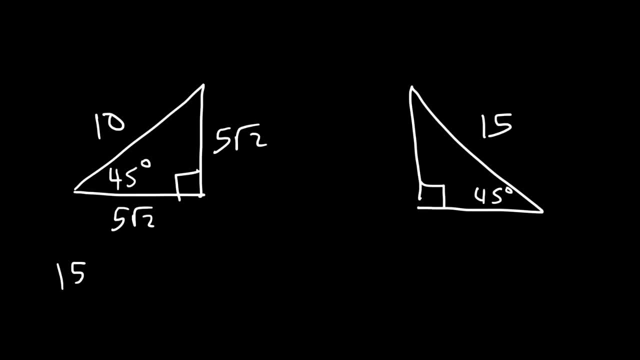 So first let's take the hypotenuse and divide it by the square root of 2.. And then let's rationalize the denominator, So in the numerator we're going to have 15 times the square root of 2.. 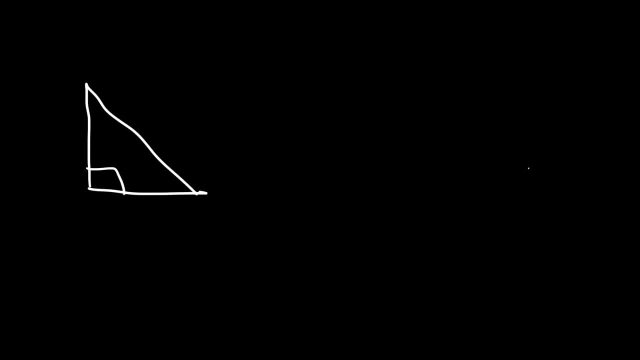 So let me give you some other examples. Let's change it up a little. So this time you're given the hypotenuse. Go ahead and find the value of the missing sides of these two triangles. Now, this time we have the side across the 90 degree angle, which is basically the hypotenuse. 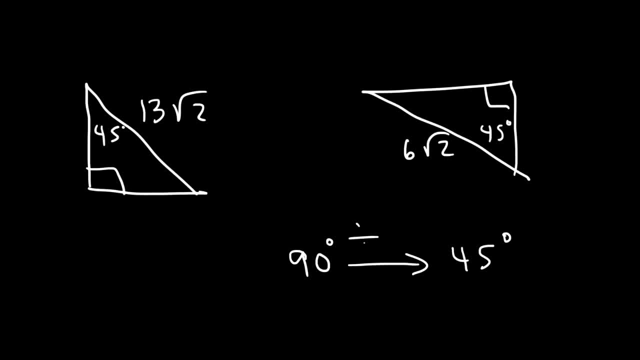 And we want to find the side across the 45 degree angle. So we're looking for the value of the shortest side. So we need to divide by the square root of 2.. So if we take the hypotenuse 13 square root 2, and divide it by the square root 2,, 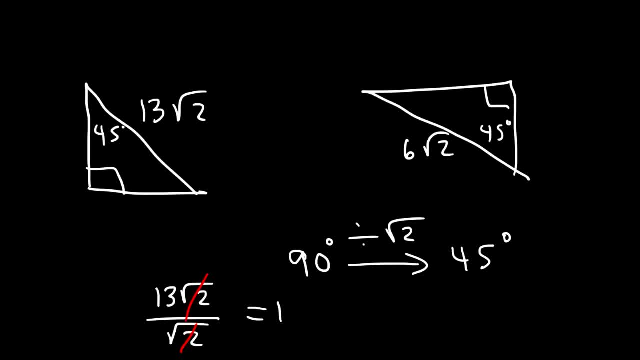 these two will cancel and we're just going to get 13.. So the length of these two sides is 13.. Now if we do the same thing for the example on the right, if we take 6 square root 2 divided by that, well, that's going to give us 6.. 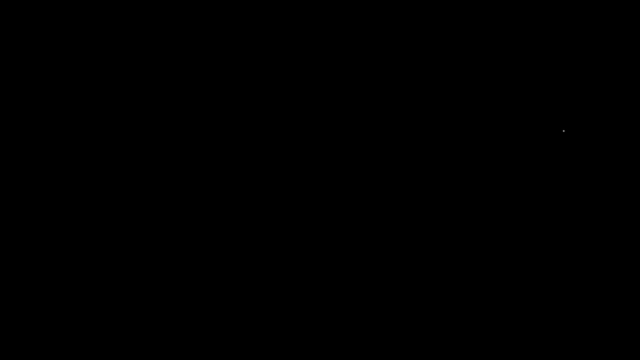 And so that's how we can easily find the value of the missing side. So consider these two examples. So let's say, this time the hypotenuse is 10, and for this one it's, let's say, 15.. Go ahead and calculate the value of the missing sides. 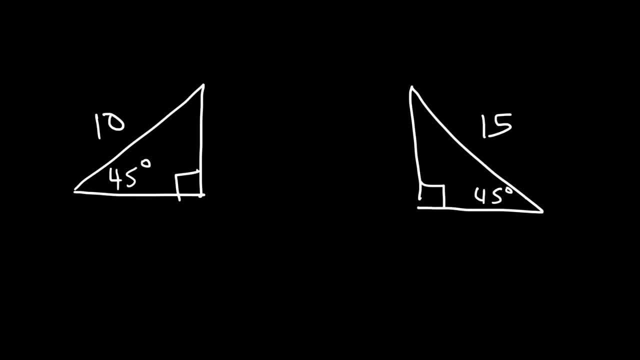 So we know, if we're given the hypotenuse to find the legs of the triangle, we've got to divide by the square root of 2.. So 10 divided by the square root of 2, is something that we need to rationalize. 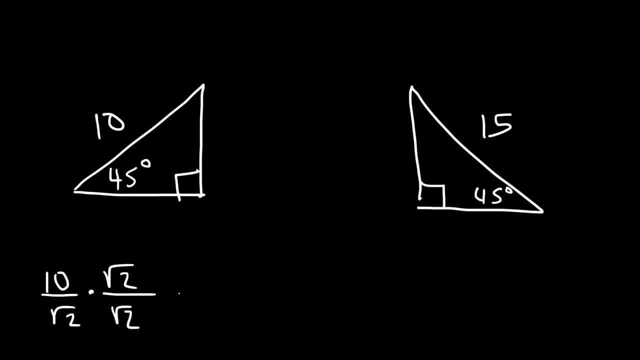 So let's multiply the top and the bottom by the square root of 2.. So on top we're going to have 10 square root 2, and on the bottom, the square root of 2 times the square root of 2 is 2.. 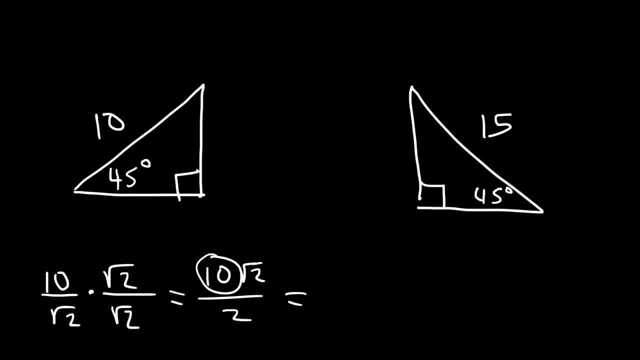 And so we could divide 10 by 2, which will give us 5.. So this is going to be 5 square root 2, and 5 square root 2.. Now let's do the same thing for the other triangle. 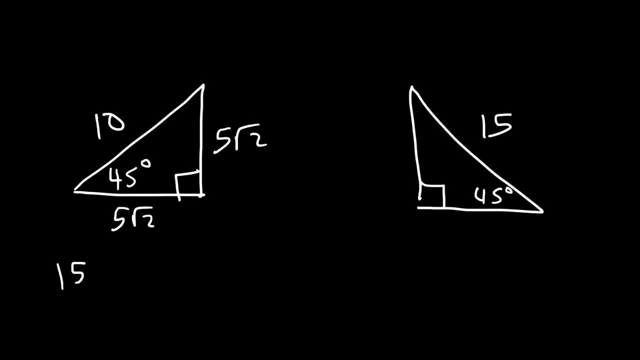 So first let's take the hypotenuse and divide it by the square root of 2.. And then let's rationalize the denominator. So in the numerator we're going to have 15 times the square root of 2, and the denominator we're just going to have 2.. 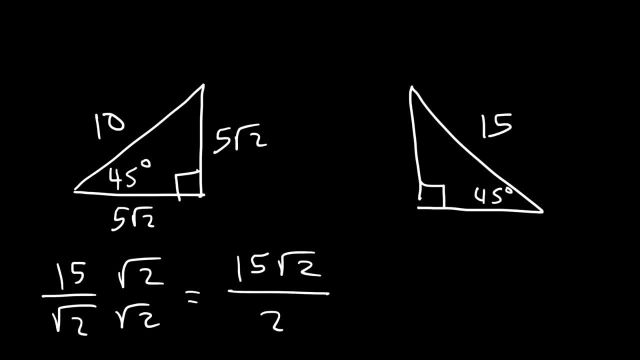 In the denominator we're just going to have 2.. Now we can't really reduce 15 over 2.. I mean you could write it as 7.5. Or you could just leave it as 15 square root 2 over 2.. 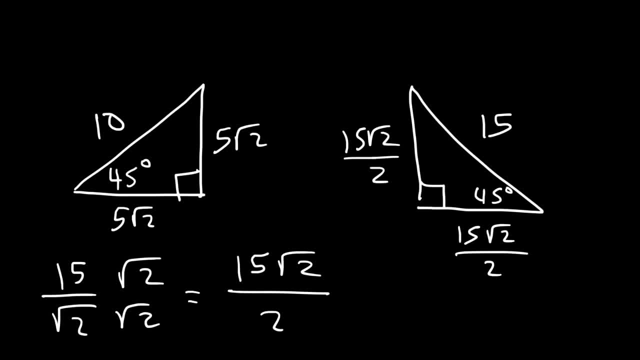 And so now you know how to solve a four-dimensional problem. So let's do the same thing for the other triangle. And so now you know how to solve a four-dimensional problem. So now you know how to solve a 45-45-90 degree triangle. 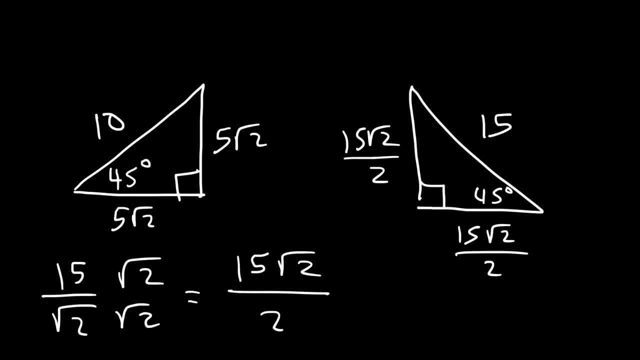 But now let's consider a practice problem that you might see on an SAT exam. But now let's consider a practice problem that you might see on an SAT exam. Let's see how we can put this information to good use. Let's see how we can put this information to good use. 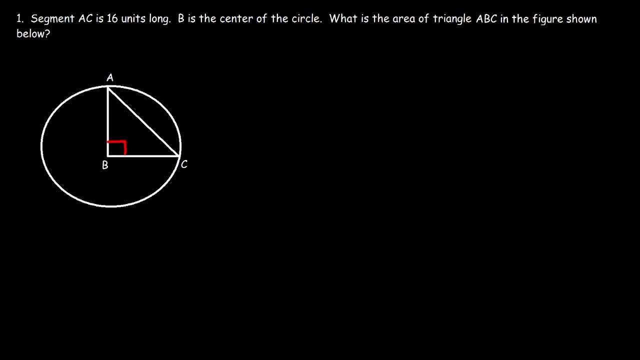 Segment AC is 16 units long. Segment AC is 16 units long. B is the center of the circle. B is the center of the circle. What is the area of triangle ABC in the figure shown below? What is the area of triangle ABC in the figure shown below? 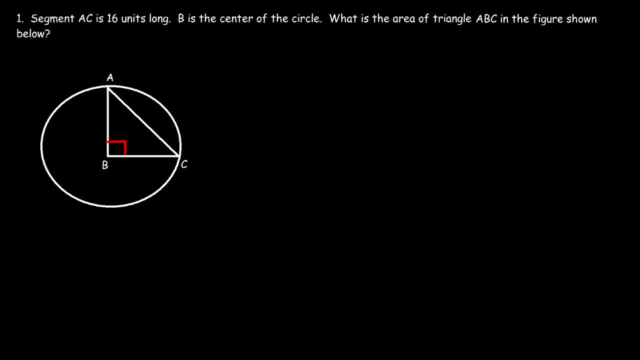 Now feel free to take a few minutes, pause the video and see if you can find the answer to this problem. Now feel free to take a few minutes, pause the video and see if you can find the answer to this problem, to this problem. Now, what kind of triangle do we have? Is it a 30-60-90? 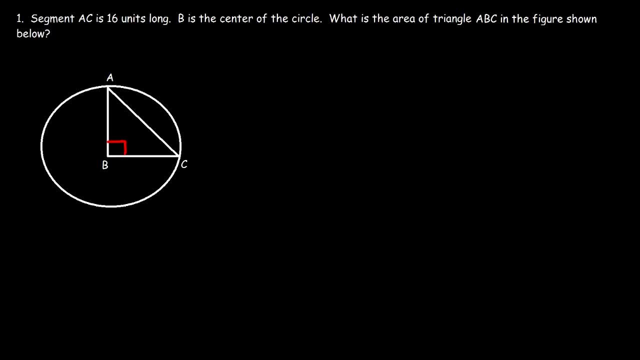 triangle or is it a 45-45-90 triangle? Since this whole video is about 45-45-90 triangles, we know that's going to be the case, But how can we be sure that it is a 45-45-90 triangle? Now, whenever you have a 45-45-90 triangle, it's important to 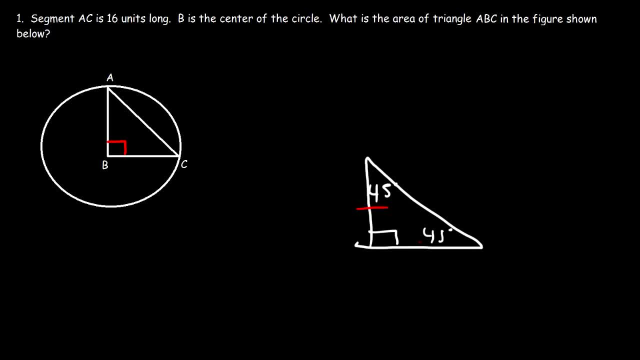 know that the sides across the 45 angles will be equal. What we have is an isosceles right triangle, And the reason why we know it's equal is because the triangle is on the circle. B is the center of the circle. The distance between 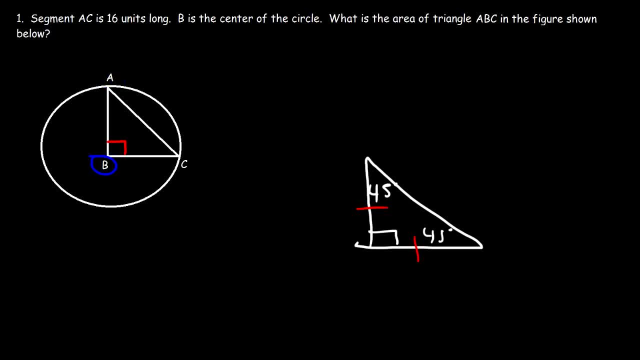 the center of a circle, and any point on a circle is known as the radius. So AB is the radius of the circle and BC is the radius of the circle, which means that those two sides must be equal To each other, And so that's how we know. we have a 45-45-90 degree triangle, So 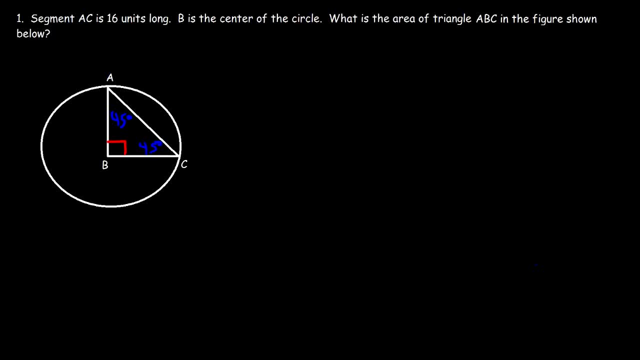 once we know that we could find the missing sides of the right triangle. Now we know the hypotenuse segment AC is 16 units long. Now to find the other sides we're going from the hypotenuse the side across the 90, to the side across the 45.. 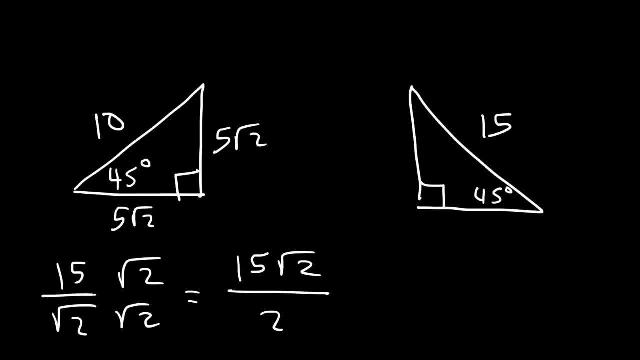 Now we can't really reduce 15 over 2.. I mean, you could write it as 7.5.. Or you could just leave it as 15 square root 2 over 2.. So that's it. And so now you know how to solve a 4x2.. 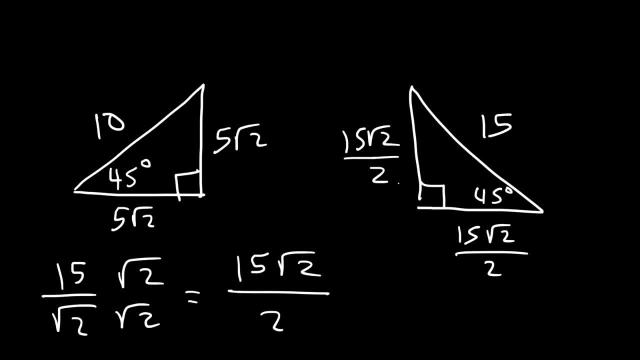 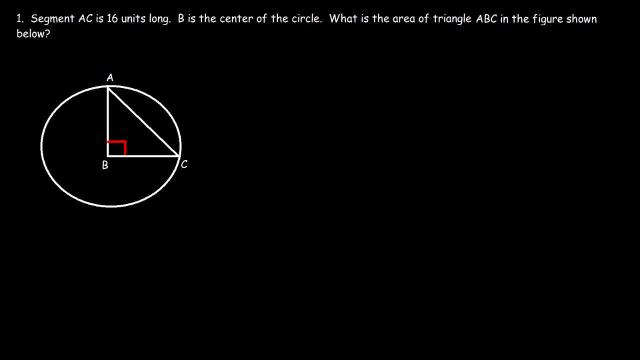 45,, 45,, 90 degree triangle. But now let's consider a practice problem that you might see on an SAT exam. Let's see how we can put this information to good use. Segment AC is 16 units long. B is the center of the circle. 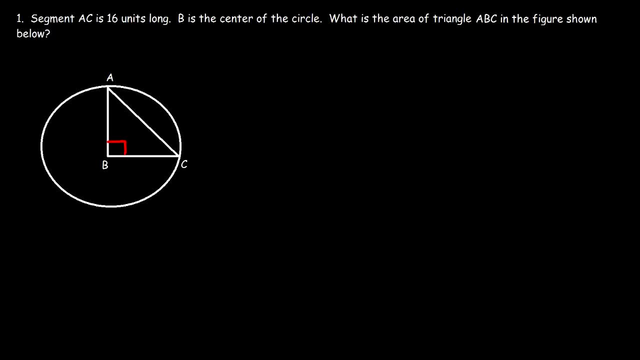 What is the area of triangle ABC in the figure shown below? Now feel free to take a few minutes, pause the video and see if you can find the answer to this problem. Now, what kind of triangle do we have? Is it a 3rd? 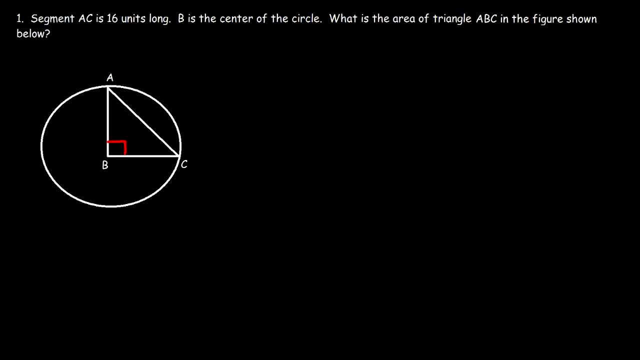 Is it a 30,, 60, 90 triangle Or is it a 45,, 45, 90 triangle? Since this whole video is about 45,, 45, 90 triangles, we know that's going to be the case. 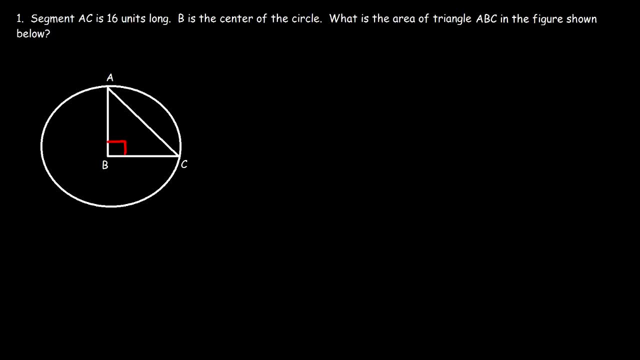 But how can we be sure that it is a 45,, 45, 90 triangle? Now, whenever you have a 45,, 45, 90 triangle, it's important to know that the sides across the 45 angles will be equal. 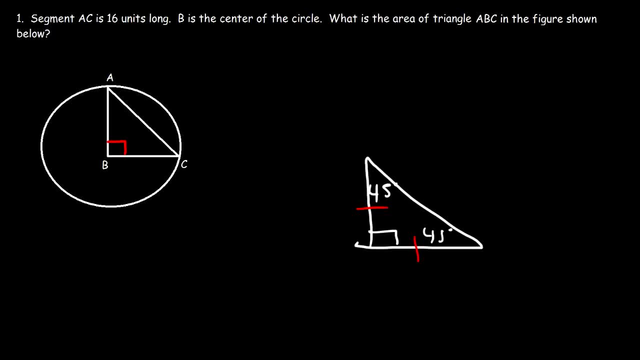 What we have is an isosceles triangle. An isosceles triangle is a 45,, 45,, 90-degree triangle. The reason why we know it's equal is because the triangle is on the circle. B is the center of the circle. 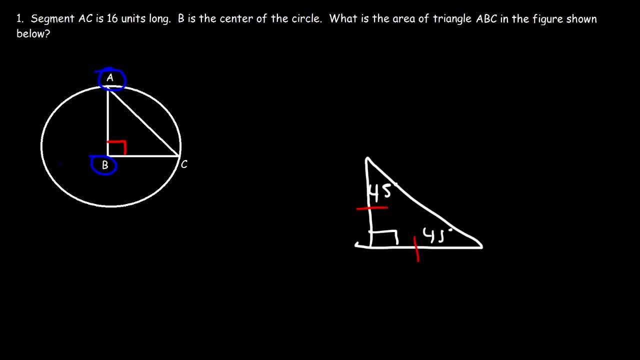 The distance between the center of the circle and any point on the circle is known as the radius. So AB is the radius of the circle and BC is the radius of the circle, which means that those two sides must be equal to each other, And so that's how we know. we have a 45,, 45,, 90-degree triangle. 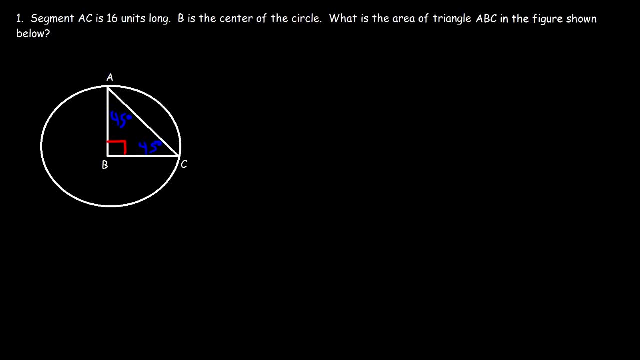 So once we know that we can find the missing sides of the right triangle, Now we know the hypotenuse segment AC is 16 units long. Now to find the other sides we're going from the hypotenuse the side across the 90, to 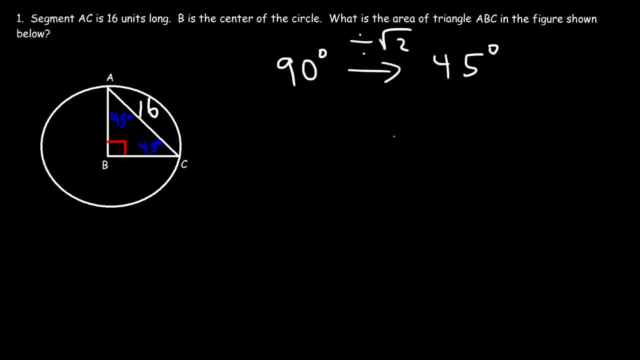 the side across the 45.. So we've got to divide by the square root of 2.. So 16 divided by the square root of 2, we need to rationalize the denominator. So let's multiply the top and the bottom by the square root of 2.. 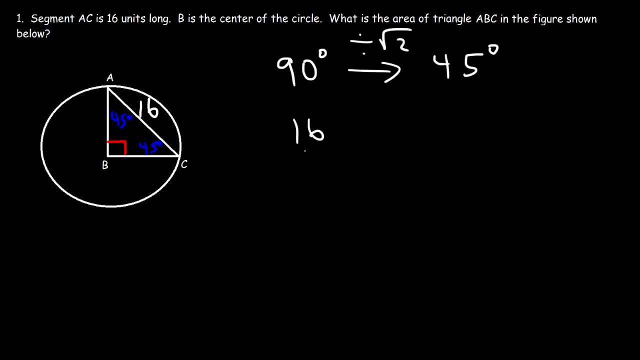 So we got to divide by the square root of 2.. So 16 divided by the square root of 2, we need to rationalize the denominator. So let's multiply the top and the bottom by the square root of 2.. So it's 16 root 2, and the square root of 2 times the square root of 2 is 2.. And 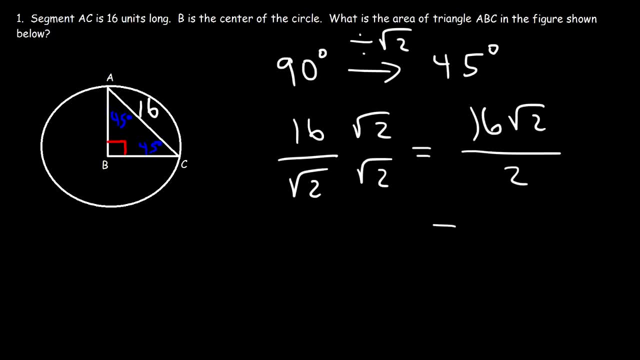 then we need to divide 16 by 2 to get 8 square root 2.. So segment BC and AB is equal to 8 square root 2.. So now that we have the base and the height of the right triangle, we can now calculate the area of that triangle. So the area is: 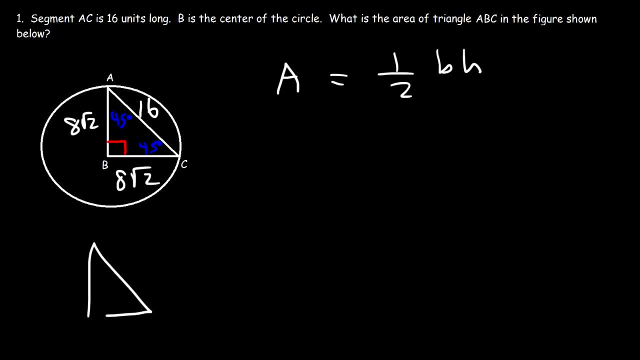 one-half base times height. So this is the base of the triangle. this is the height, So it's going to be one-half. We have a base of 8 square root 2 and the height of 8 square root 2.. So first let's multiply 8 by 8.. 8 times 8 is 64.. Next, 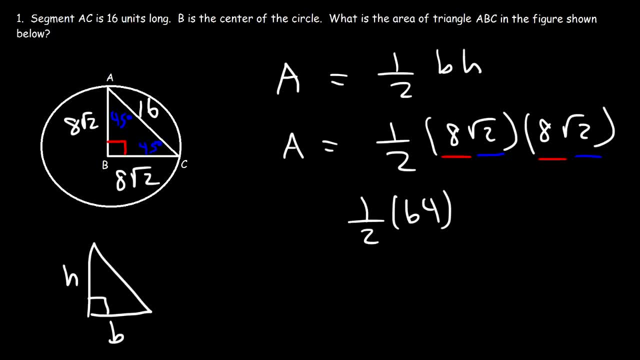 let's multiply the square root of 2 times the square root of 2, which we know to be 2.. Now, one-half times 2 is 1, so we could cancel those two. So the area of triangle ABC is 64 square units in value. So this is the answer to the. 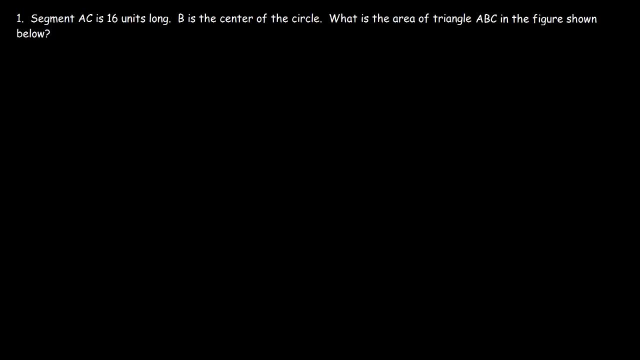 problem. So that's basically it for this video. Hopefully you found it to be useful. Now you may want to check out my next video on 30-60-90 special right triangles. So I'm going to have some problems like this one, which can help you for the SAT and the HT exam at least. 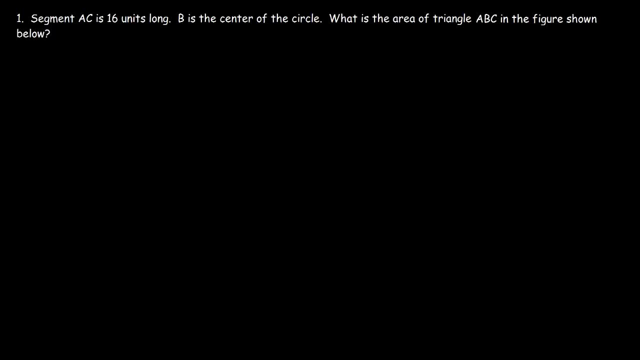 the math sections for those exams. So just keep this in mind Whenever you're dealing with a 45-45-90 triangle. if you have the side across the 45 and you want to find a side across the 90 or the hypotenuse, multiply by the square root. 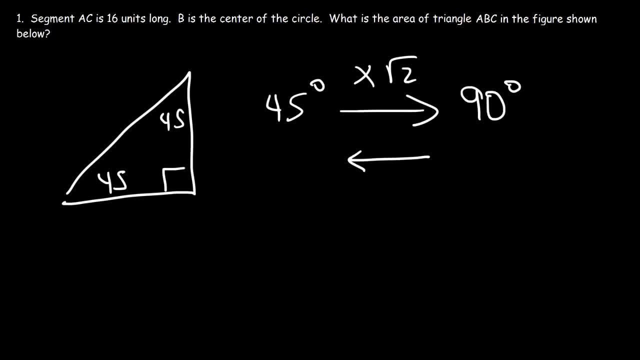 of 2.. And if you have the hypotenuse and you want to find the length of the legs of the triangle, or basically the side length across the 45-degree angle divide by the square root of 2. If you remember this, you can mentally find the answer. 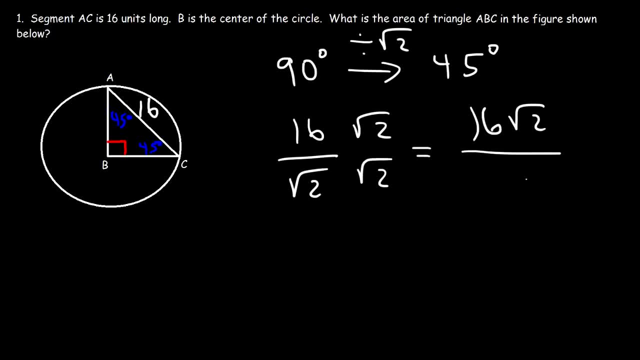 So it's 16 root 2, and the square root of 2 times the square root of 2 is 2.. Then we need to divide 16 by 2 to get 8 square root 2.. So segment BC and AB is equal to 8 square root 2.. 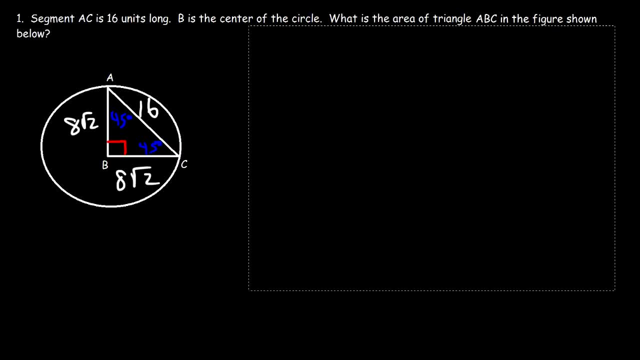 So now that we have the base and the height of the right triangle, we can now calculate the area of that triangle. So the area 8 is 1 half base times height. So this is the base of the triangle, this is the height. 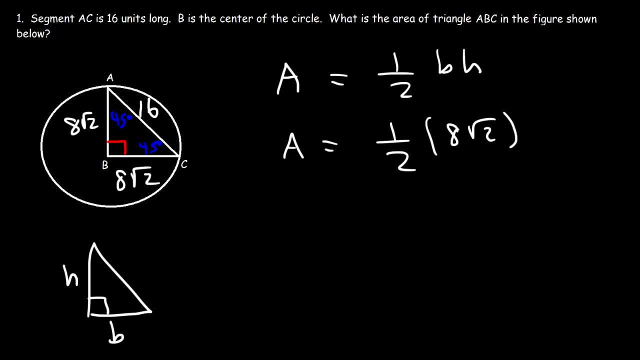 So it's going to be 1 half. We have a base of 8 square root 2, and the height of 8 square root 2.. So first let's multiply 8 by 8.. 8 times 8 is 64.. 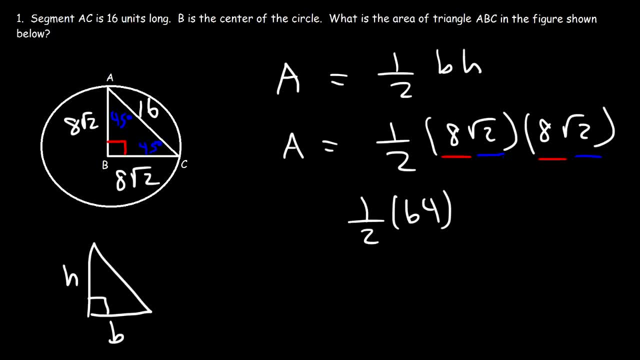 Next, let's multiply the square root of 2 times the square root of 2, which we know to be 2.. 1 half times 2 is 1, so we can cancel those two. So the area of triangle ABC is 64 square units in value. 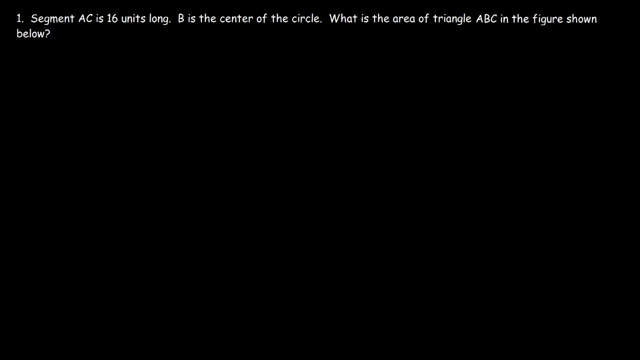 So this is the answer to the problem. So that's basically it for this video. Hopefully you found it to be useful. Now you may want to check out my next video on 30-60-90 special right triangles. So I'm going to have some problems like this one. 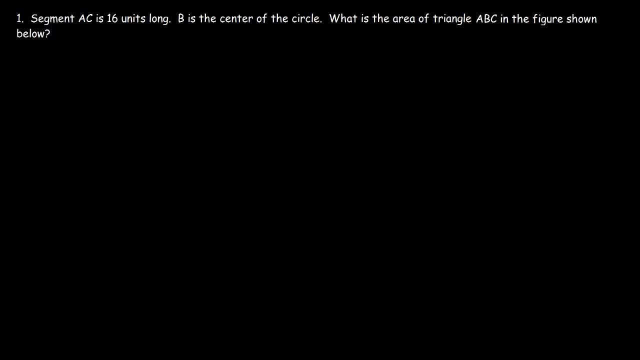 Which can help you for the SAT and the ACT exam, at least the math sections for those exams. So just keep this in mind Whenever you're dealing with a 45-45-90 triangle. if you have the side across the 45, and you 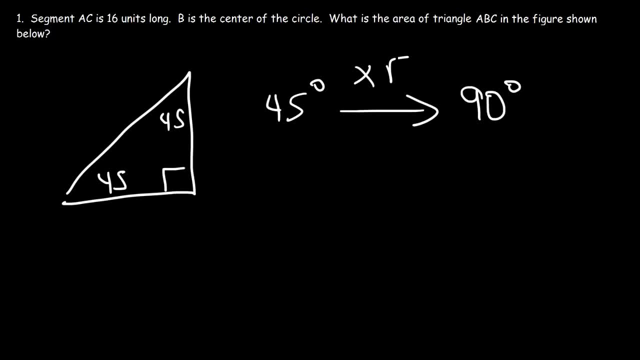 want to find the side across the 90, or the hypotenuse, multiply by the square root of 2.. And if you have the hypotenuse and you want to find the length of the legs of the triangle, or basically the side length across the 45 degree angle, 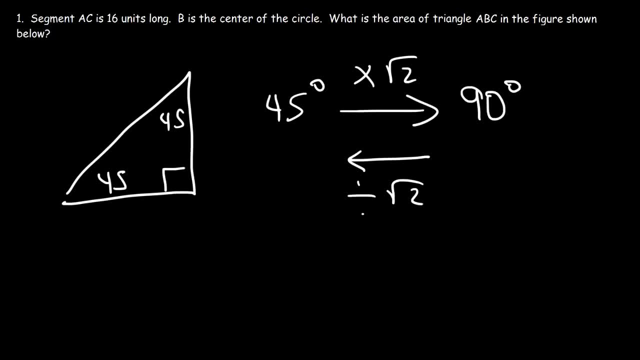 Divide by the square root of 2.. If you remember this, you can mentally find the answer in your head. It can save you a lot of time, especially when you're taking the SAT exam, because you got to get the answers quickly. You can't waste time.